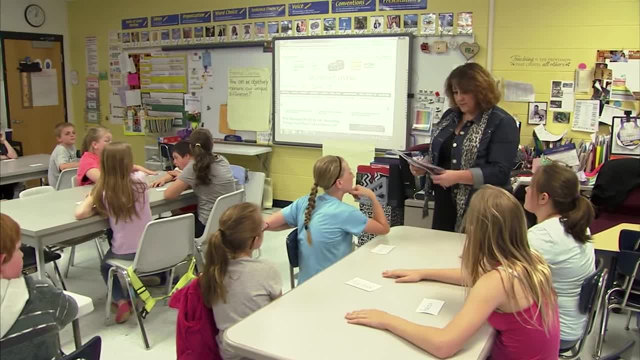 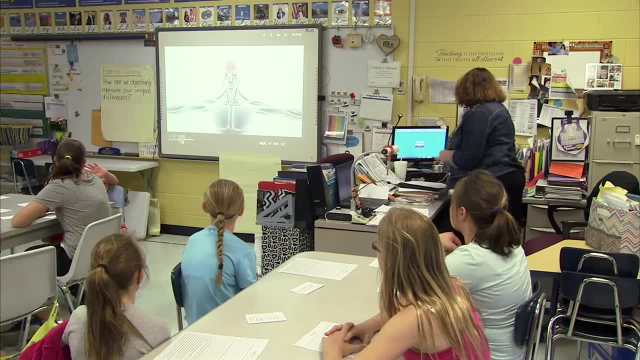 and then we're going to be able to measure some things about our body as well. My name is Chrissy Wheeler and I teach at Village of Barbersville Elementary School in Barbersville, West Virginia, and I teach fifth grade. It's the human body in numbers. 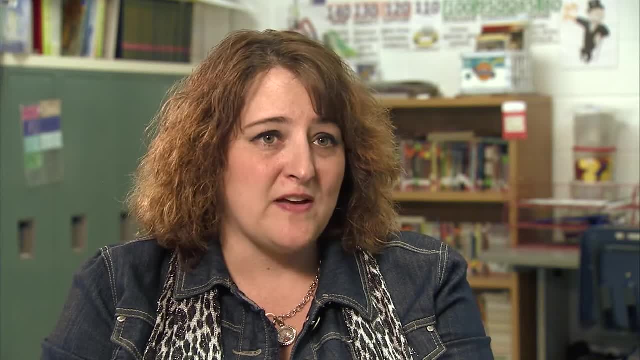 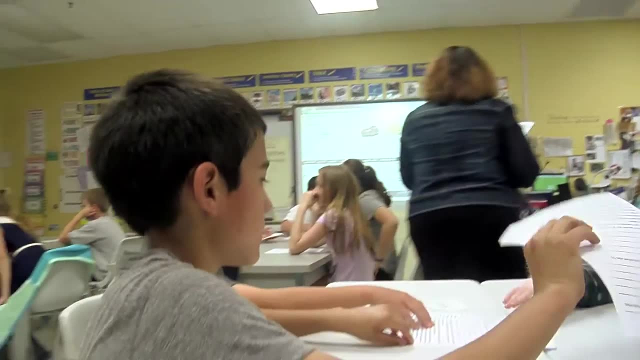 This lesson is about measurement. Students often have a hard time with metric measurement in the intermediate levels, So, as I was planning this lesson, I started with a content that I knew I already had to cover, that students needed a lot of help with, And so measuring their bodies was a great shift to this. 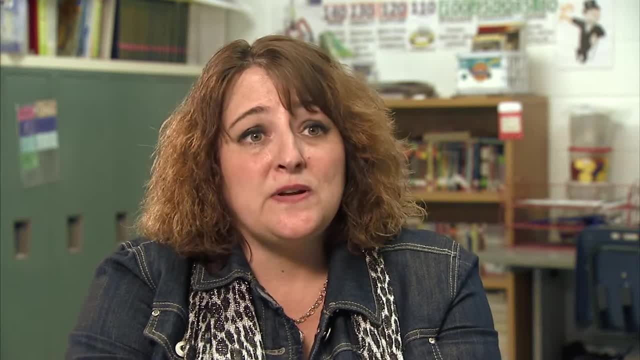 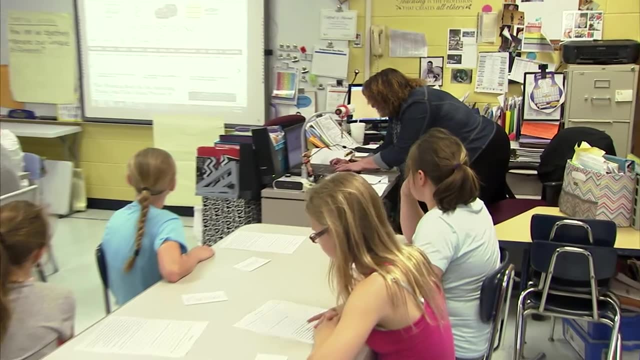 and a great culminating activity, and incorporating Kahoot and Office Mix and the Rulers app was a really easy way to just deepen the understanding with metric measurement for the students. So we're going to watch a very short video clip and I want you to think about what you notice about your body. 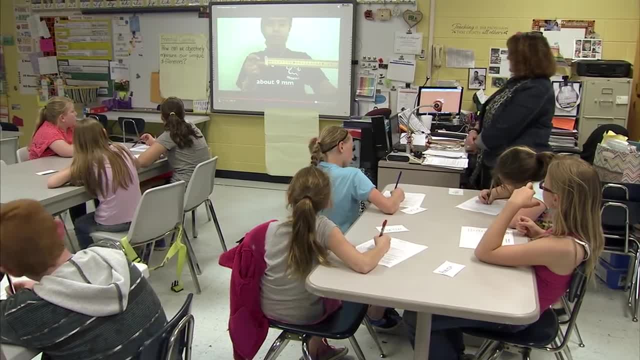 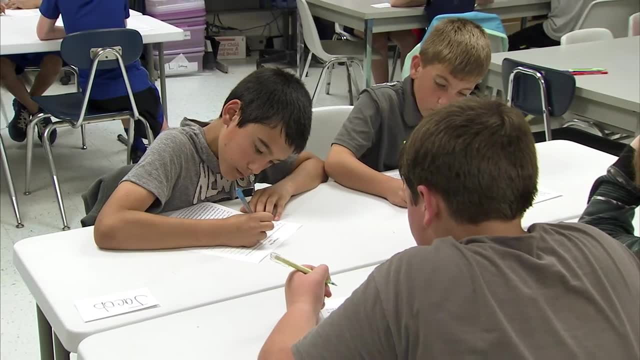 Okay, in the hook of the lesson the students are watching a video to get them hooked and one of them is about how unique they are. So it talks about numbers in the body that are just astronomical, that students haven't thought about before. 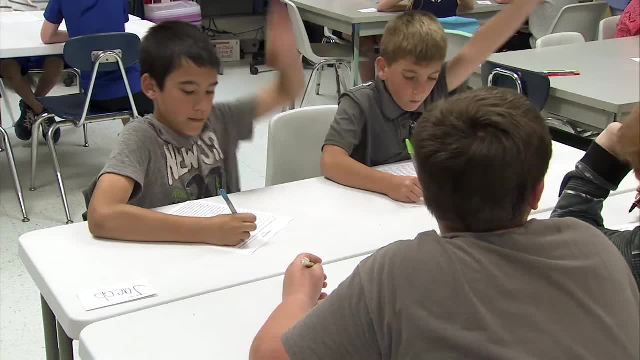 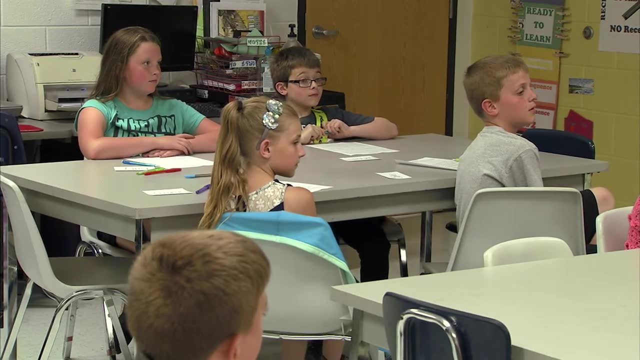 Okay, who can give us one fact that they notice that makes their body special? That we shed 620 grams of skin every year. Good, Alright, so we're going to take a formative assessment to see what we know about estimating how big something is. 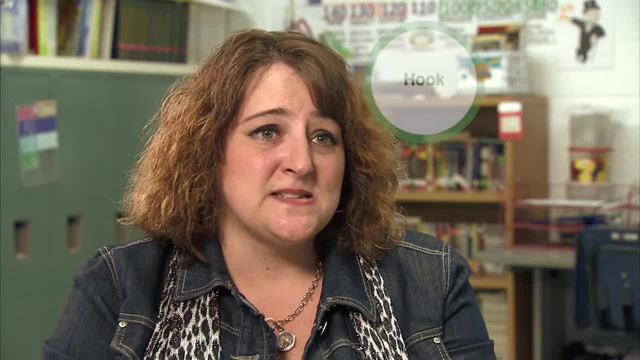 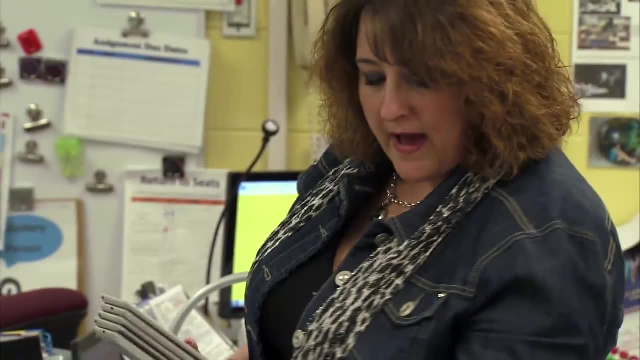 We also will be using the Kahoot app so that students can see if they're good at estimating and also think about their body parts and how long each of those pieces would be on them. So go ahead and when you get your computer, go onto Kahoot like we did earlier. 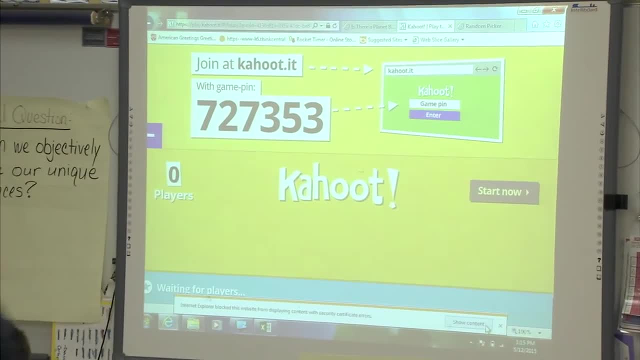 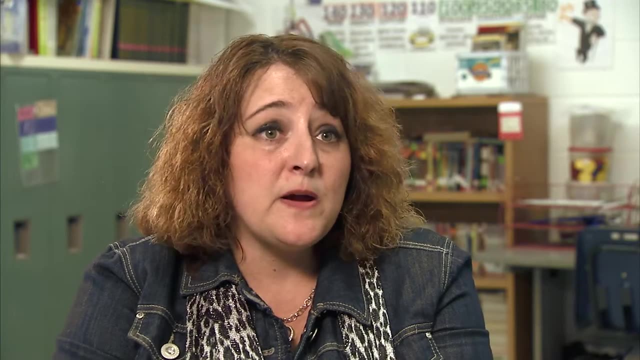 To meet my learning goals. I wanted to make sure that we weren't just using apps or technology just for fun, that it had a purpose, and so I feel like the ones that we chose were very purposeful, for what we did. Is the average length of your face greater or less than 7 inches? 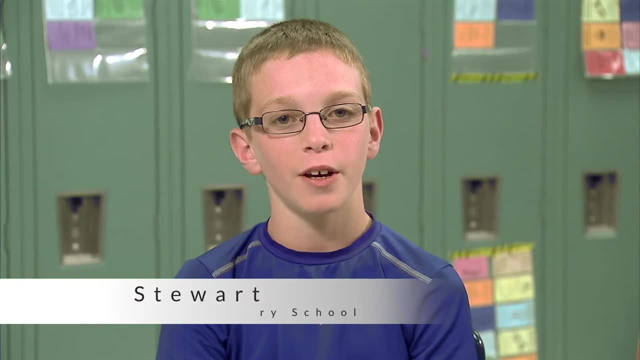 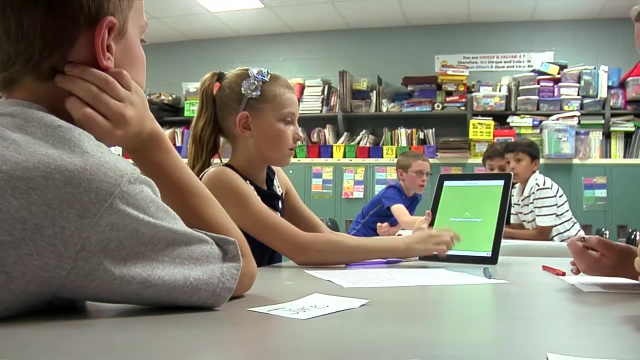 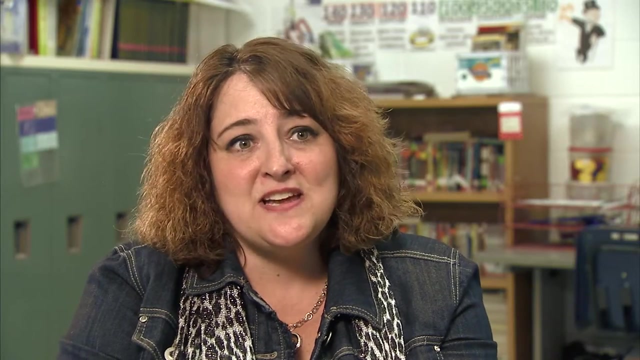 I really like using other tools, especially Kahoot, because that makes it really competitive and I'm pretty competitive at a lot of things. Yes, I love using the Kahoot app Because they're so competitive and it makes them pay attention and they really want to win and get the answers right. 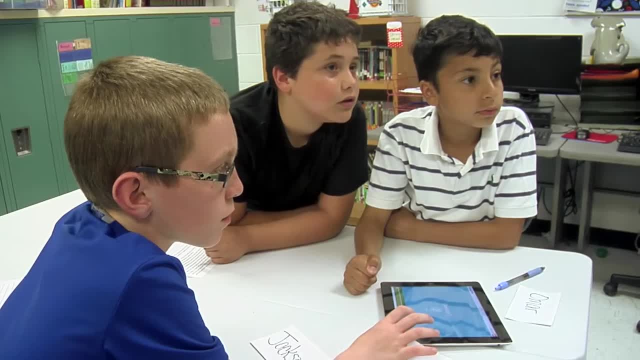 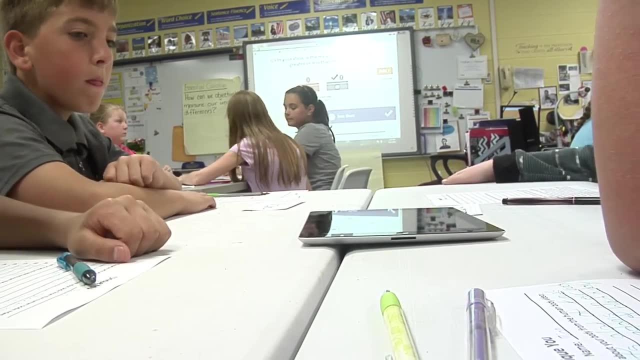 and it's a good review for them as well. Is the average length of your ear greater or less than 2 1⁄2 inches Less? I think it's very important that we incorporate technology as much as possible, and so, if I can do that within my lessons, that's what I do. 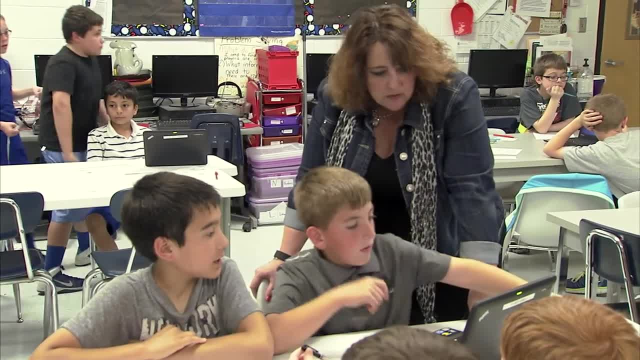 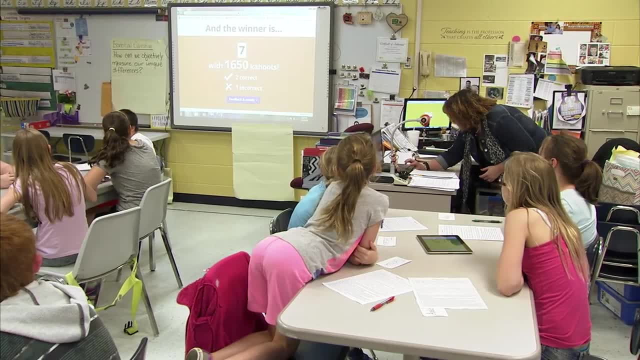 I try to come up with lessons that I know I have to cover and then see where I can embed the technology in there without it being just fluff or something extra that we do. All right. so now what we're going to do is we're going to talk about how to measure correctly. 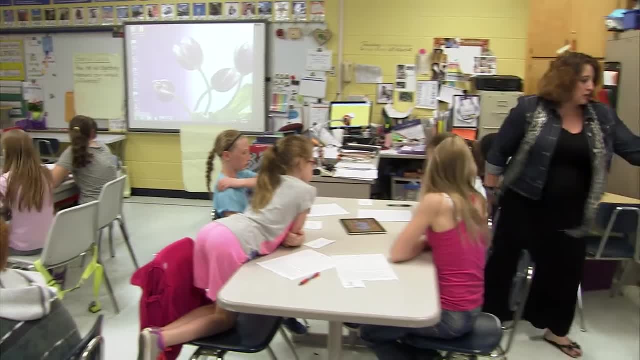 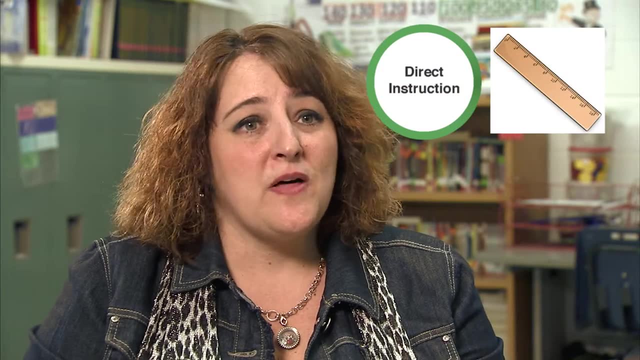 Who can remind us how we measure with a ruler or a measuring tape, the right way. So for direct instruction, we are going to use centimeter rulers and I'm going to put them on the Elmo document camera so that the students can see the proper way to measure. 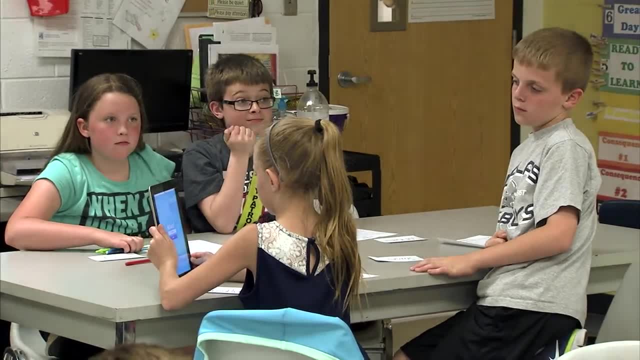 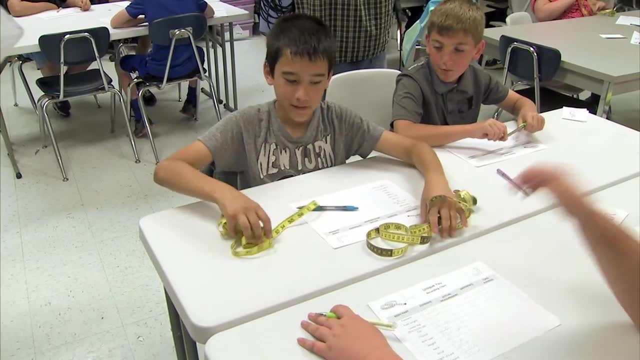 so that they start at the zero, so that they get accurate measurements. And I'm going to give you just a couple of minutes to take a couple of objects and measure them. Okay, Find three things to measure, Three things For guided practice. we are using an app called Rulers. 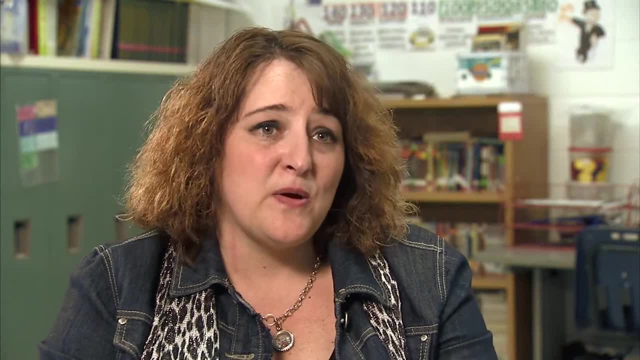 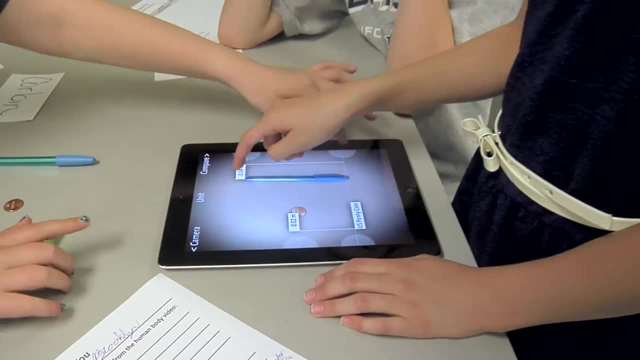 and the students can take everyday objects like pennies or iPhones or pens or whatever they have available and they can estimate what they think the lengths will be and they take a screenshot of it and then they are using those to compare other objects to. 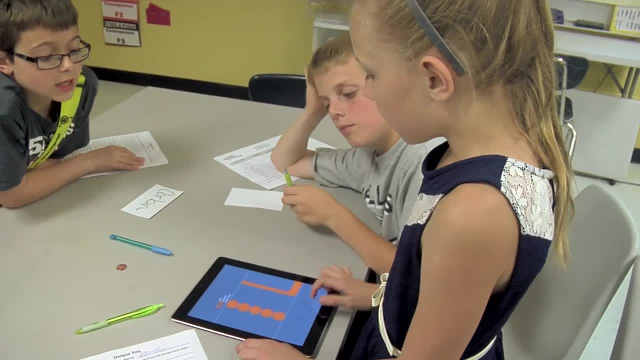 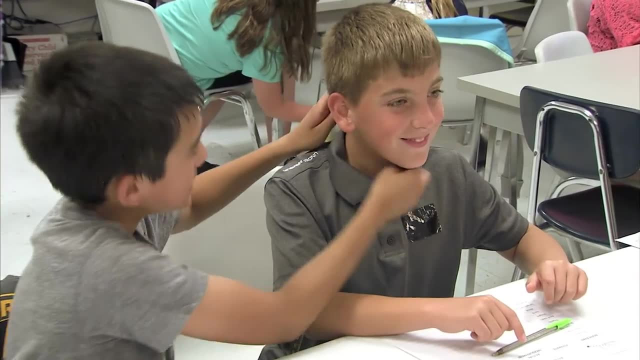 So they can see if they're good at estimating it. I thought it was going to be eight. For independent practice. the students are partnering up and they are going to measure each other's bodies And then they can compare that to their estimates. 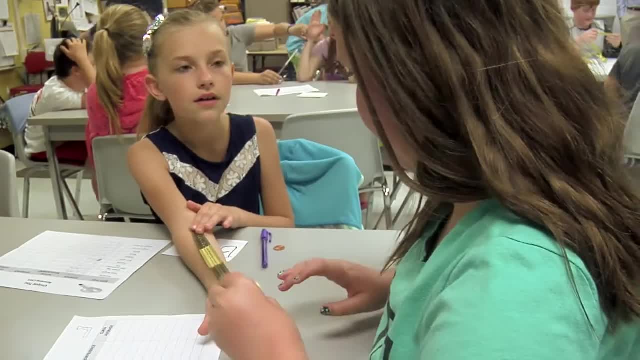 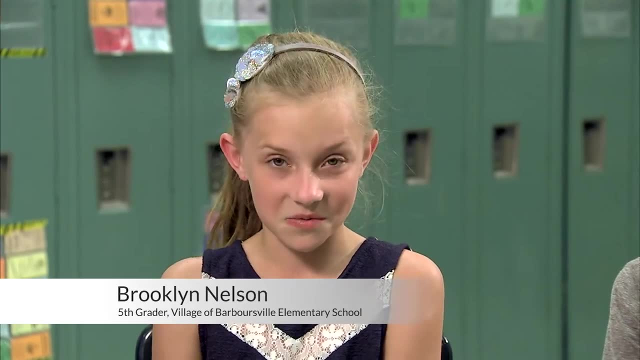 to see how good they were at estimating. That was 35.. 35. I said 30. My favorite part of the lesson was where we got to work with our partners and it was fun to know that when you measure your arm span. 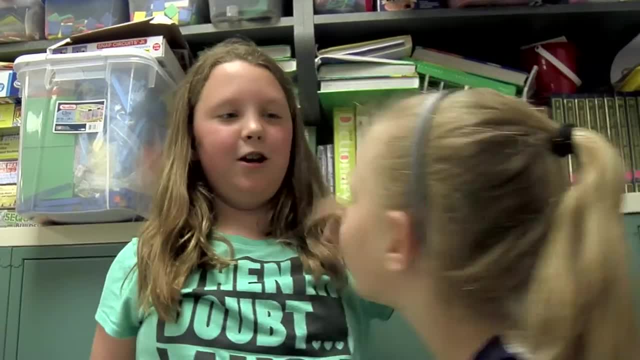 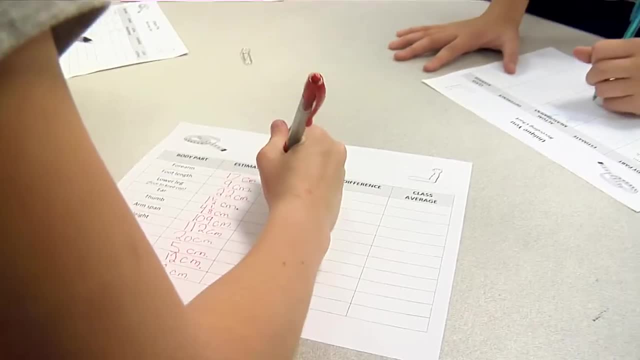 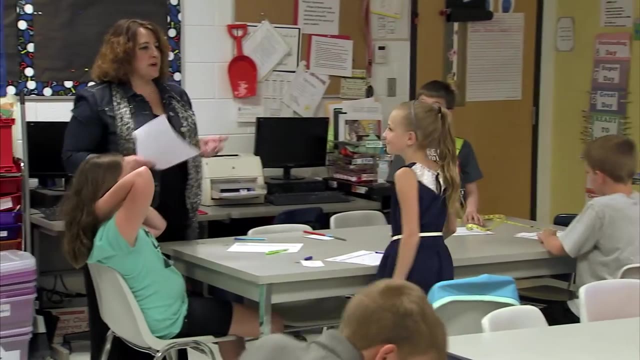 then you know: oh, that's my height, Four more So 154.. 21.. Oh my gosh. Oh, that's the same as I got Two-minute warning. How many of you now think you're a good estimator in what we just did? 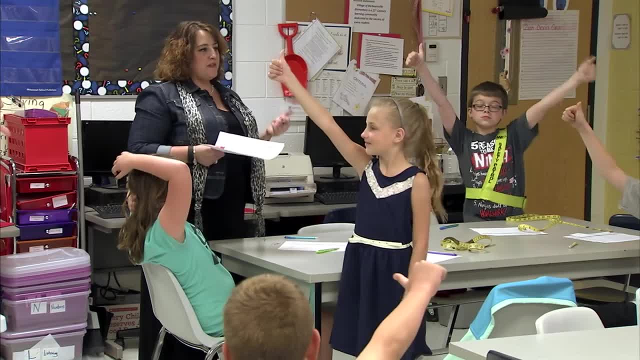 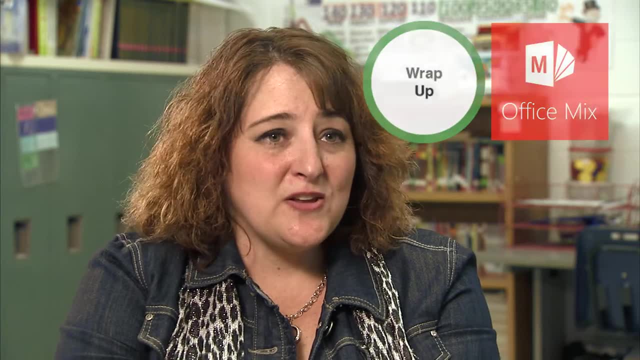 or not so good. you need some practice. Thumbs up if you think you did pretty well. For the wrap-up, the students use Office Mix, which is embedded in PowerPoint, and so that they can use that to see what attributes were similar. 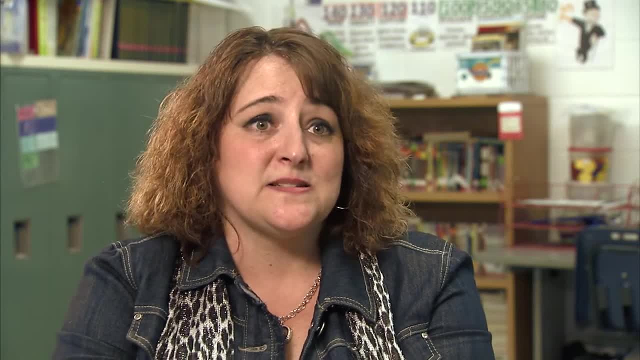 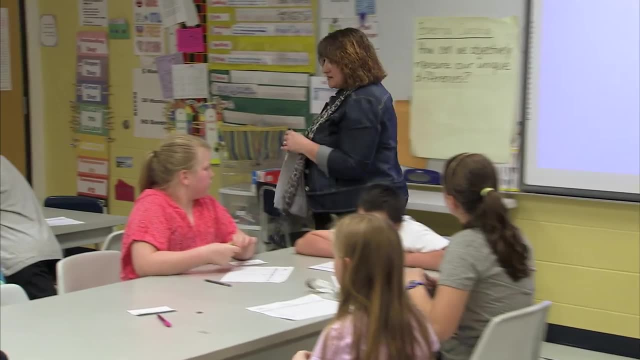 within their actual measurements during the independent practice. You know you have to have a title page, maximum of three slides, and one of them has to incorporate Office Mix in there. Have one of you log in so you can go ahead and get started. 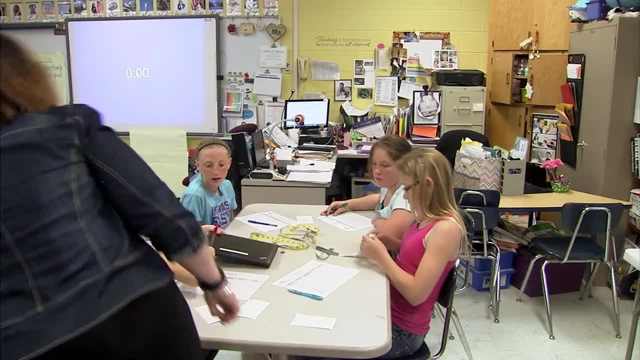 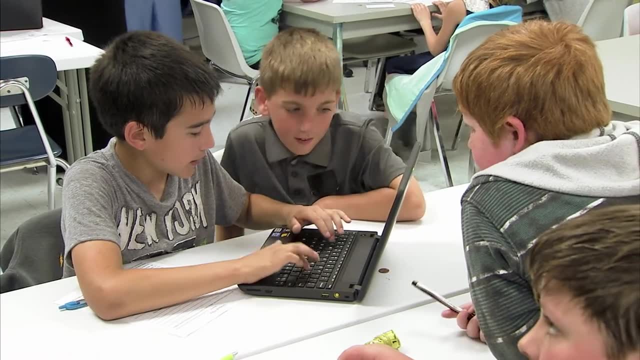 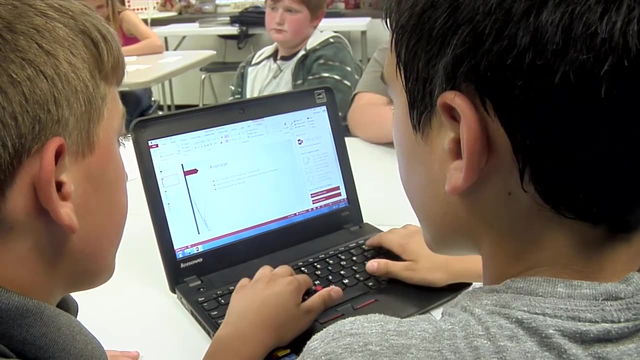 The rest of you can be. you all can be just asking what you're going to put on there. My favorite part of the lesson is probably when we were learning about Office Mix and we were doing it together in groups, because this way, like since, there's more than two people. 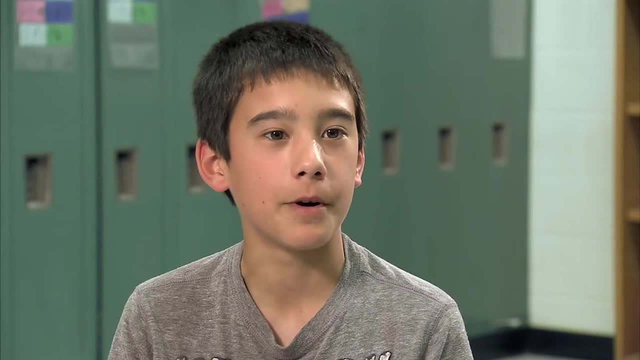 if someone wasn't doing their share of work, then it wouldn't just be one person doing it. If someone was doing all of it, it could be maybe two or three out of like four. Okay, so we're going to wrap up. 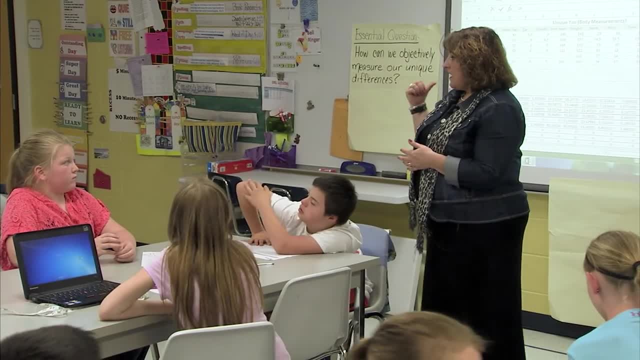 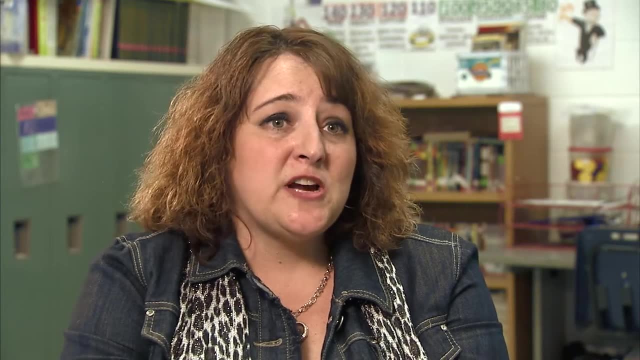 and we're also going to find the rest of the class average for our each of our body parts and see how the class average compares. For the wrap-up, the students also share out to the class so that the class can see all the different attributes. 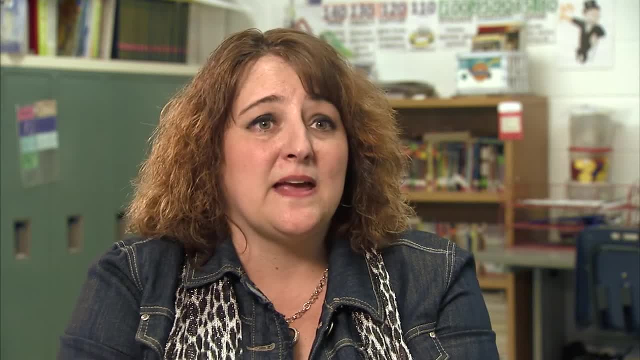 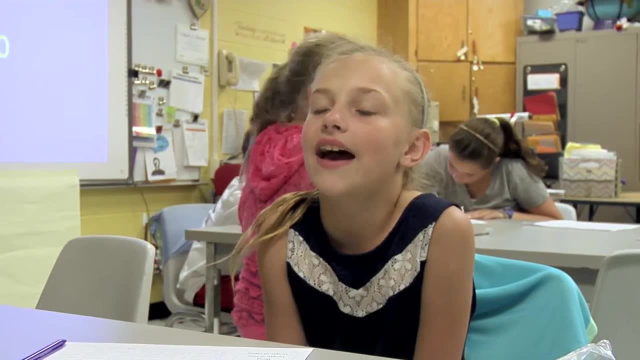 and what characteristics their body parts had that made them unique and the relationships between the body parts. I noticed that my height was the same as my arm span. I noticed that, you know, my hand is about the length of my face and that's kind of weird. 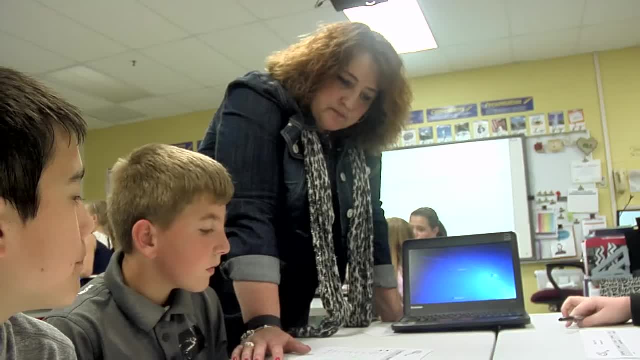 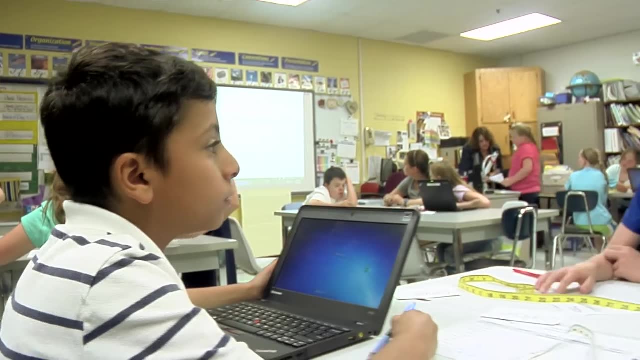 We have so many digital learners now, and we have to, as educators, be able to reach them on the level that they are on at that moment, and so we have to be creative and be able to incorporate technology into our lessons. What do you see as a relationship? 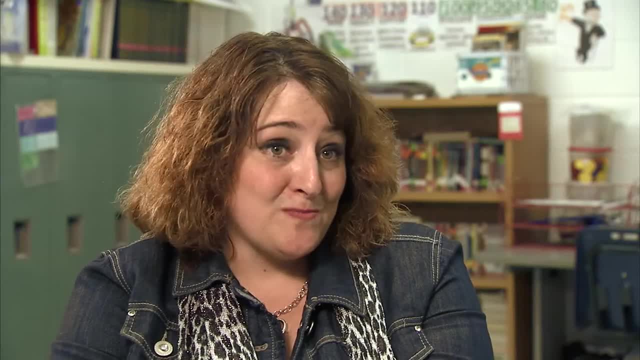 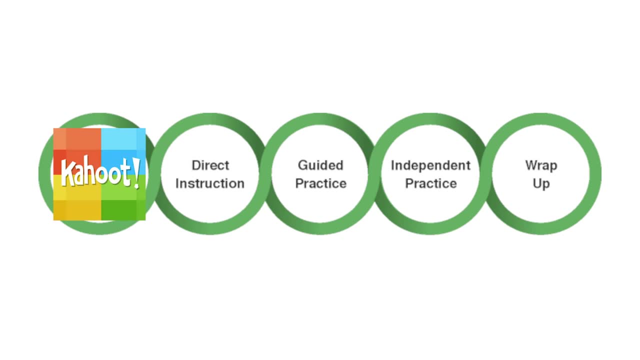 The tips that I would recommend for teachers would be to start small. I think that if you start with a lesson that you already do in class and then if you can just embed technology in it, maybe just in one area or something that the students are already comfortable with. 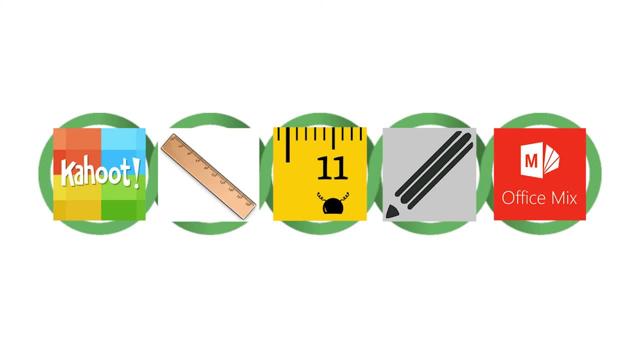 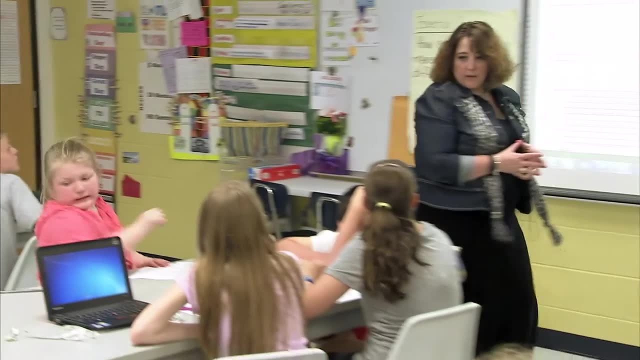 or that you as a teacher are comfortable with. then I think you'll be more willing to try other things and step outside the box the next time to incorporate other technology tools into your lessons. So I want you to shut computers down. If you have started on yours, go ahead and save it. Captions by GetTranscribedcom.